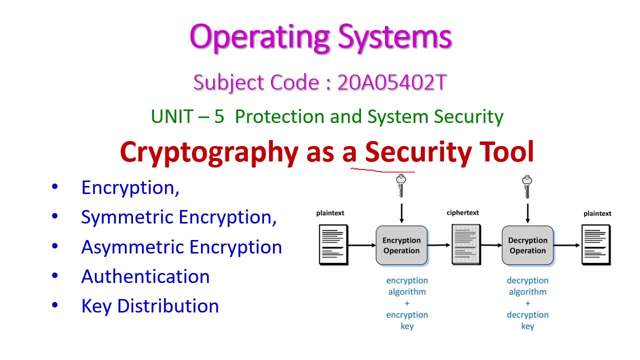 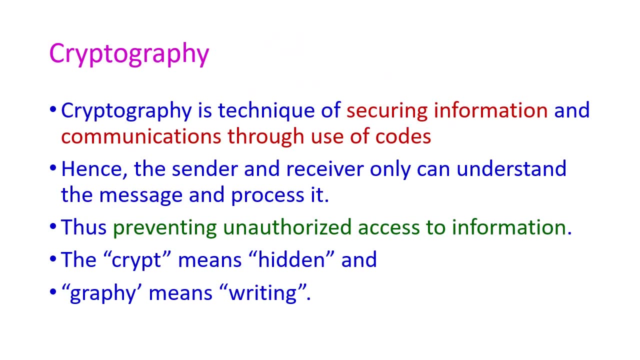 In this operating system class, we will see the cryptography as a security tool and under this topic, we will see the encryption and the two types of encryption, that is, symmetric and asymmetric encryption. After that we will see the authentication and key distribution. First, let us see what is cryptography. It is a technique of securing information and communication through use of codes, Hence the sender and receiver only can understand the message and process it. 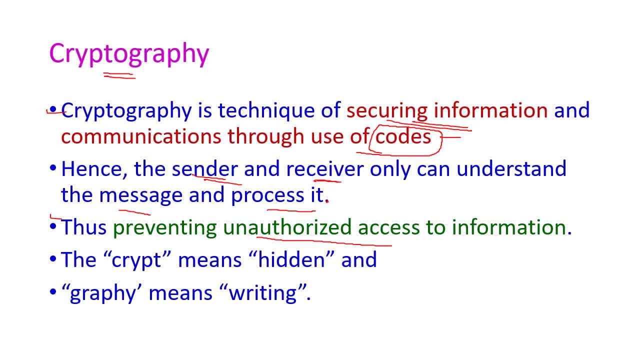 OK, thus preventing unauthorized access to the information. OK, here, crypto means hidden and graphe means writing, Hence cryptography means hidden writing. Cryptography is actually the sender is here and receiver is here. The sender is going to send a message that is a very big, normal message and that will be given to the receiver. 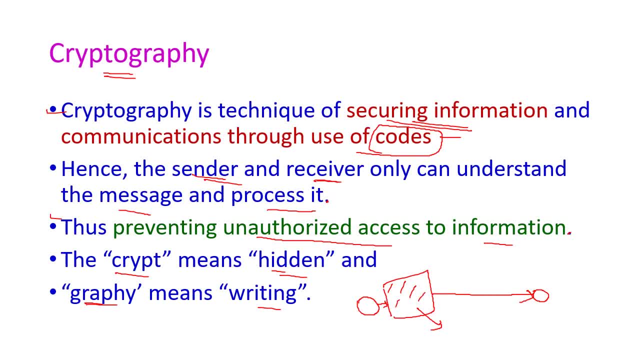 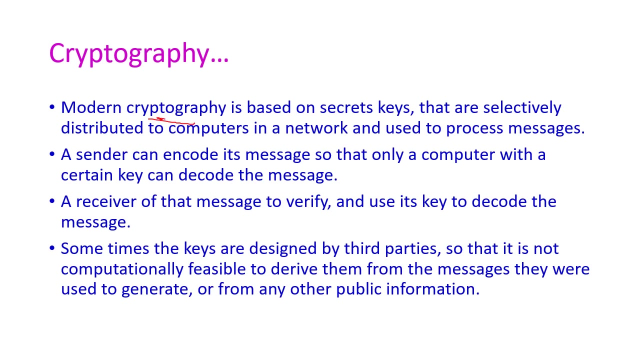 But in this original normal message, some secret is hidden in this message and only this sender and receiver can understand the secret. The other person cannot find any difference in these messages. Okay, so this is called as cryptography. In modern cryptography, it is based on secret keys and the keys are selectively distributed. 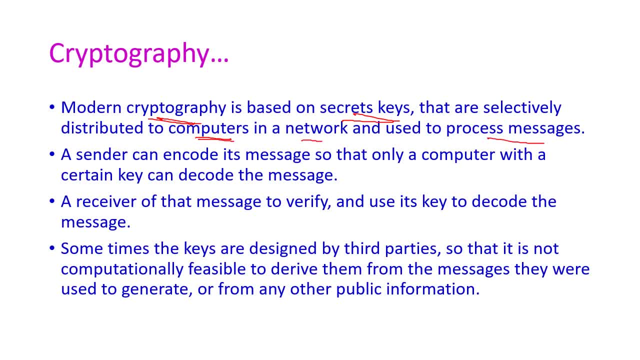 It is distributed to computers in the network and used to process the messages. That is, the sender and receiver are connected through the network. Through the network, the sender and receiver are connected and sorry, this is receiver. The sender is having its own message and they are having a key for sender. Okay, by using the key, the sender will encrypt his message and the encrypted cyber text will be transmitted to the receiver. 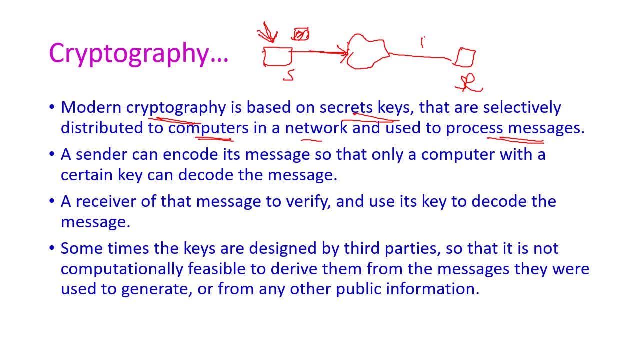 To the internet and the receiver will receive this encrypted cyber text and the receiver will use his key to decrypt this particular message. Okay, then the receiver will get the plain text. that is the original text. Okay, right, The sender can encode its message so that only the computer with certain key- who is having this key the receiver is having isn't it To decode the message? Okay, the receiver can decode the message by using the key. 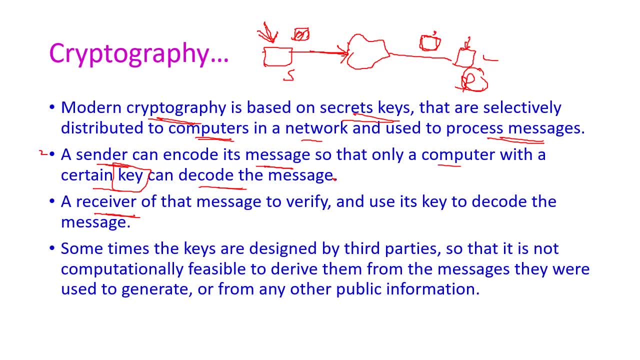 Receiver's key and receiver of the message to verify and use its key to decode the message. Okay, this is what this particular scenario and sometimes the keys- that is, the secret keys- are designed by third parties, So it is computationally not feasible to derive from the message, that is, from this message, which they are used to for communication. 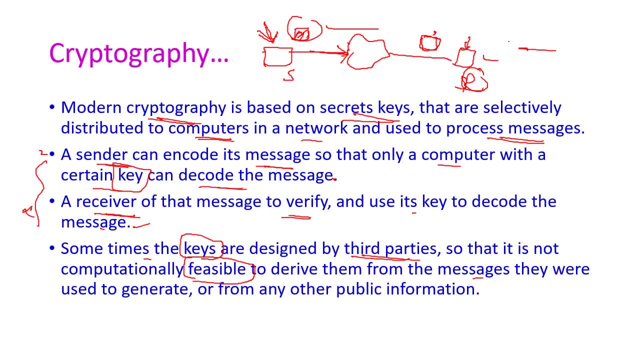 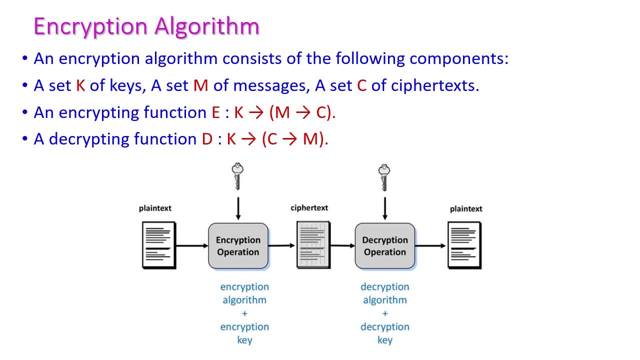 Or these keys are not possible to take from the public information. Okay, this is the cryptography, And next let us see the working of encryption algorithm. It consists of a set of keys and a set of messages and a set of cyber text. Okay, here the sender and the receiver are going to share the code. 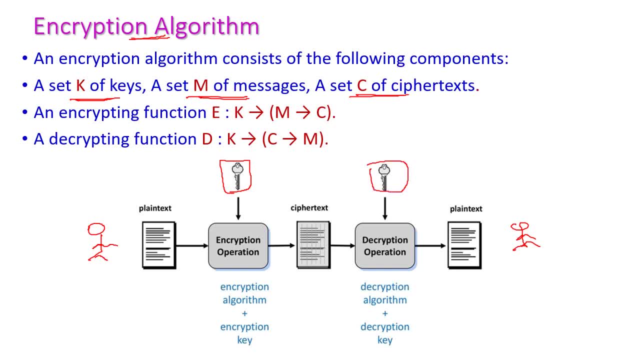 A common key. Okay, this is called us key. That is k. Okay, is representing this key. The key will be shared between sender and receiver. That is, these two systems will be connected in the Internet and a common key will be shared between sender and receiver. Okay, first of the plain text, That is the secret messages having by sender And the secret message will be encoder. Okay, that is the secret message is sending the same type of message. Please understand that this is. 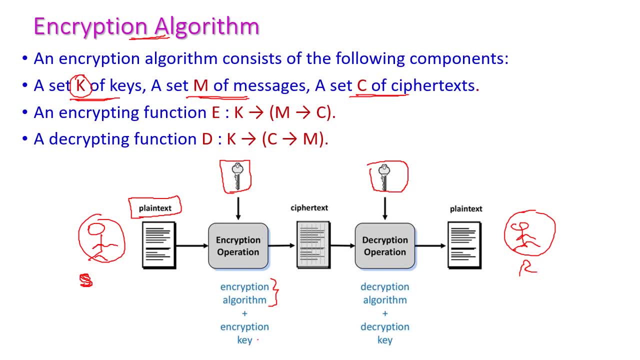 by using the encryption algorithm with the help of encryption key. After this encryption operation, the output will be ciphertext. Only the ciphertext will be transmitted from sender system to the receiver system In the internet. only the ciphertext will be transmitted from sender system to receiver system. 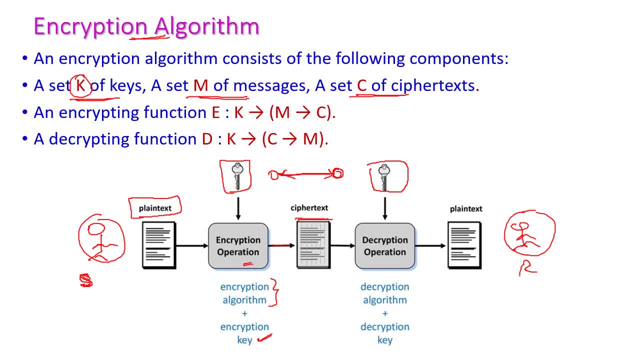 When come to receiver end, the receiver will receive the ciphertext and he will use this decryption operation, that is, decryption algorithm, with the help of decryption key. The key will be shared between sender and receiver. After this decryption operation, the receiver will get the plain text, which is actually the secret message. 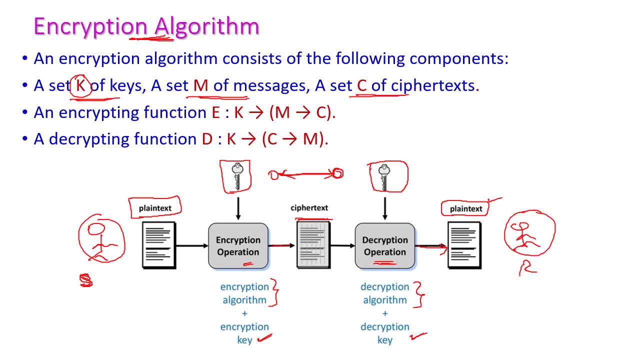 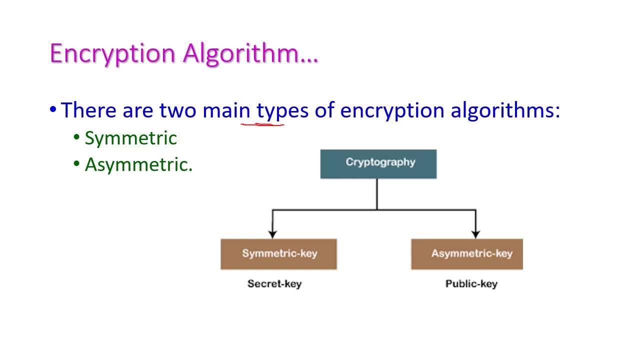 This is how the encryption algorithm is working. There are two types of encryption. First one is symmetric encryption and second one is asymmetric encryption. In the symmetric encryption, the same key will be shared between both sender and receiver. When come to asymmetric encryption, different keys will be shared between sender and receiver. 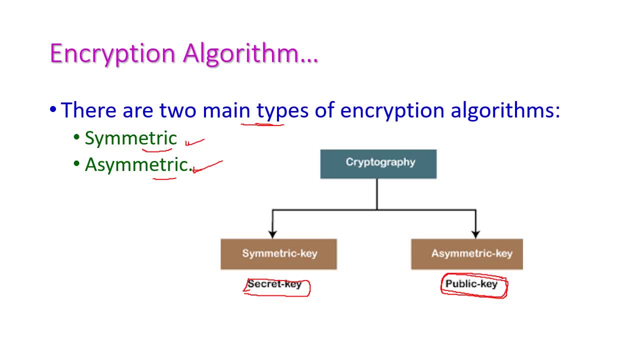 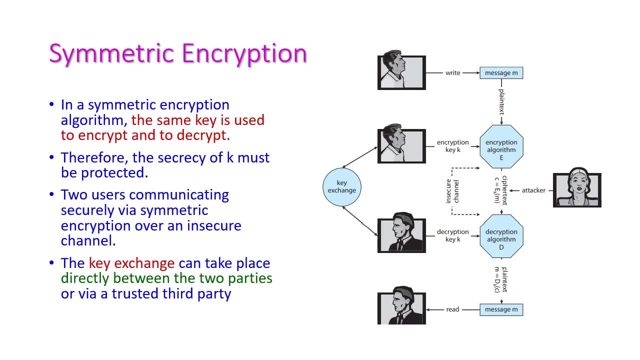 Encryption will be taken place by public key, but decryption will be taken place by a separate key, which is the receiver is having Symmetric encryption, As I already told you, a same key which is used for both encryption as well as decryption. See first, this is the sender side and this is the receiver side. 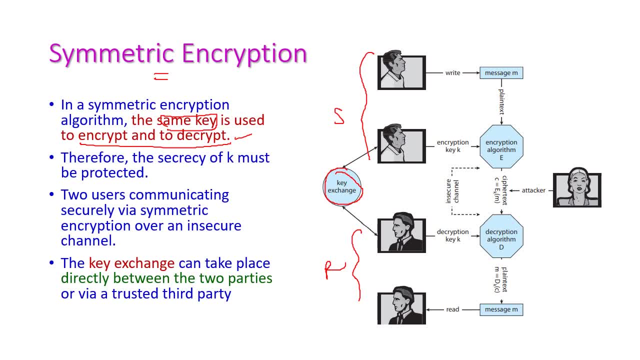 So a same key will be exchanged between the sender as well as receiver. So the sender is having a plain text. The plain text will be encrypted by using encryption algorithm with this key, Then the encrypted key, That is the cipher text. 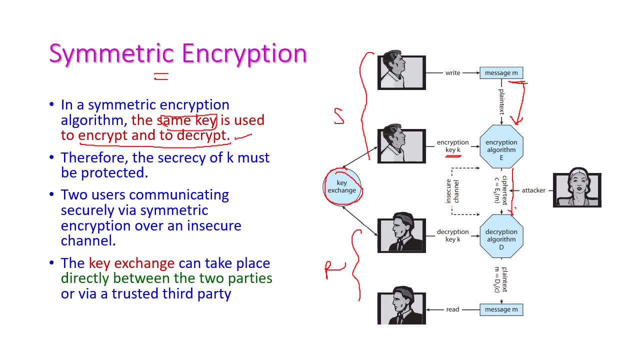 That is, the encrypted text, will be transmitted in the internet. Actually, the attacker is going to track this particular channel to get the information, But the information is actually encrypted now Encrypted information. So there is no use of the encrypted message with this attacker. 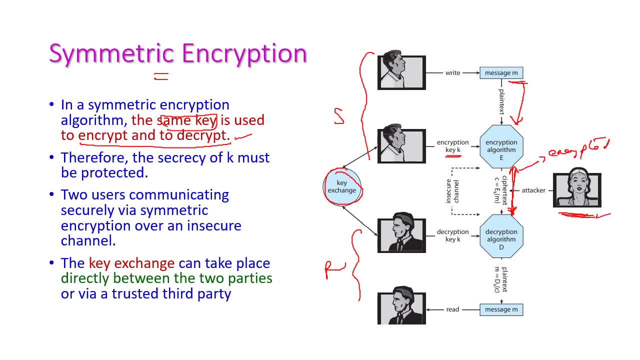 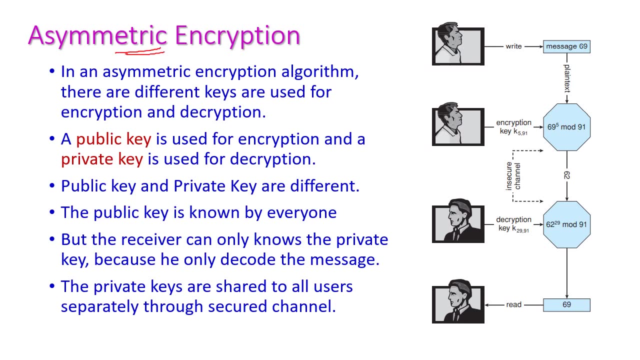 Right. When come to receiver side, the receiver will use the same key For decrypting this particular cipher text. then the plain text will be given to the receiver. When come to asymmetric encryption, different keys are used for both encryption as well as decryption. 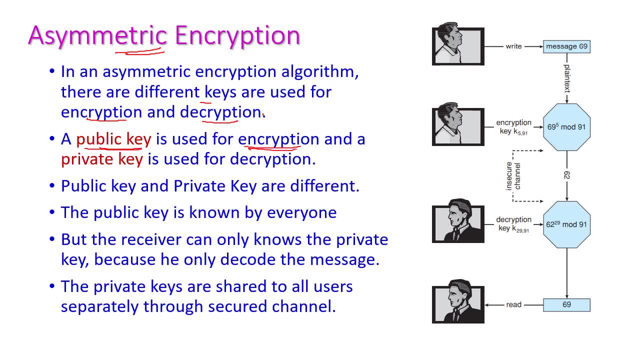 Okay, Here the public key is used for encryption and the private key is used for decryption. Okay, That is, the sender will use public key for encrypting the text And the receiver will use his own private key for decrypting that text. 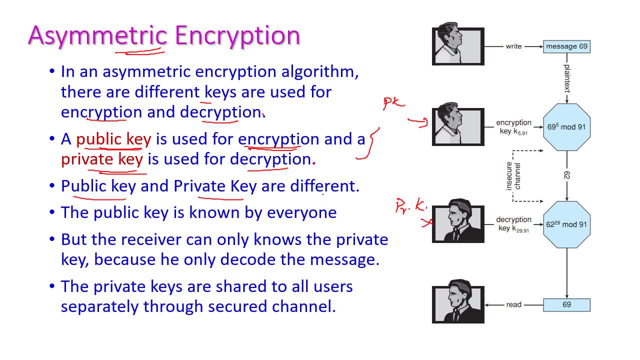 Okay, See, public key and private key are different. Okay, And public key is known by everyone who are connected in the network, But the receiver only knows about his own private key. Okay, Private key is secret key, that each and every user have its own secret key. 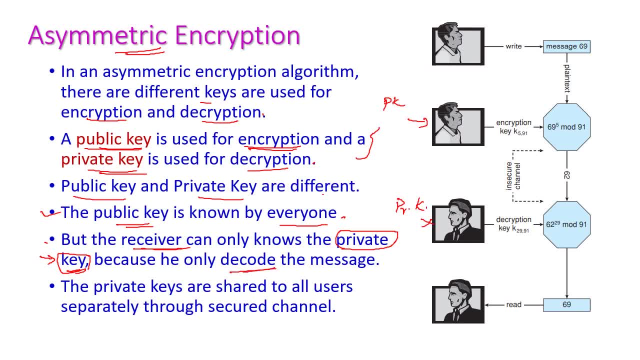 Right, Because the receiver only decode the message. Right Here, public keys and private keys will be shared to all the users who are connected in the network separately through a secured channel. Right, This is asymmetric encryption Here. see, this is the sender side. 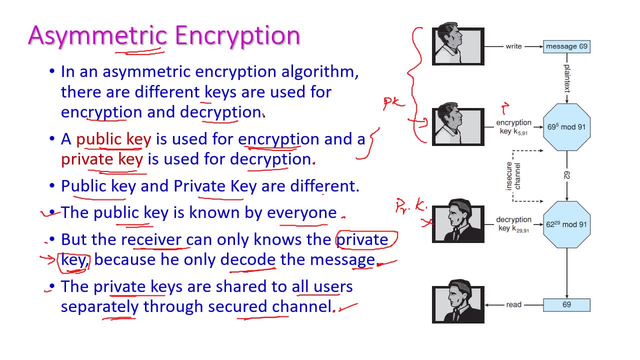 The sender will use the public key. PK means public key, Okay, Public key for encrypting, And at east of the server, the sender'. Now it was sent to all the users of the BOMU and status. So this is output for BOMU and Selenium. 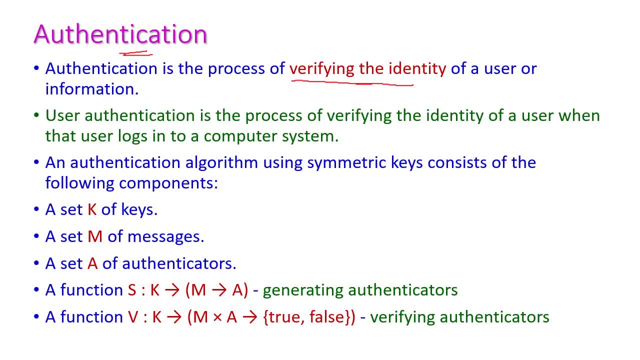 Yes, sir, It is also callable sir. Yes, Okay, Thank you so much. identity of a user or the information the user authentication is a process of verifying the identity of a user when that user logs into the computer system. okay, see, when a user logs into. 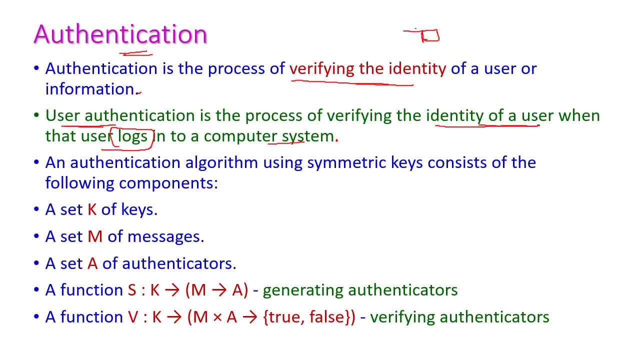 a computer system, then immediately we need to verify whether the user is authorized user or not. okay, so this is called as authentication. okay, here, authentication algorithm using symmetric keys which consist of following components. which are the components? a set of keys, a set of messages and a set of authenticators. okay, and it is also having two functions. the first function is yes, which is: 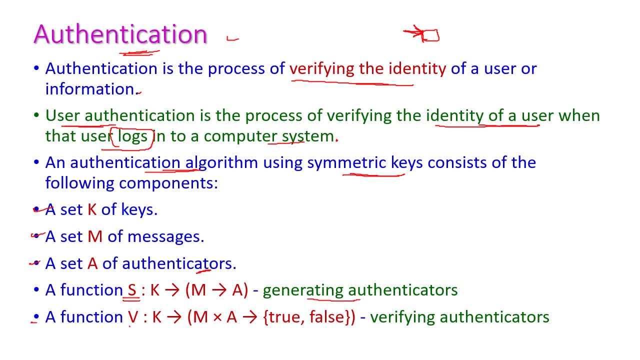 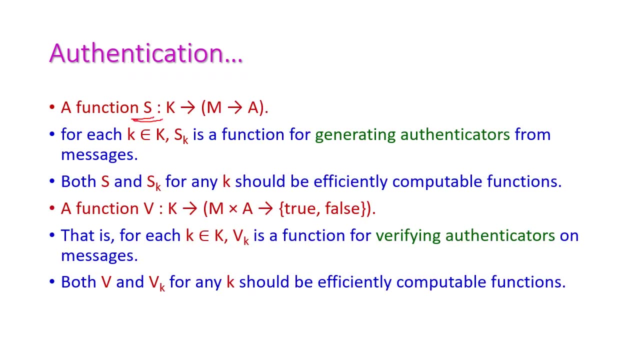 for generating the authenticators, and second function is v, which is for verifying the authenticators, whether the user is authorized user or not authorized user. the first function is: yes, this function is used to generate the authenticators from the messages. okay, that is, our users are connected to the internet. okay, in the net, for all users we have to give. 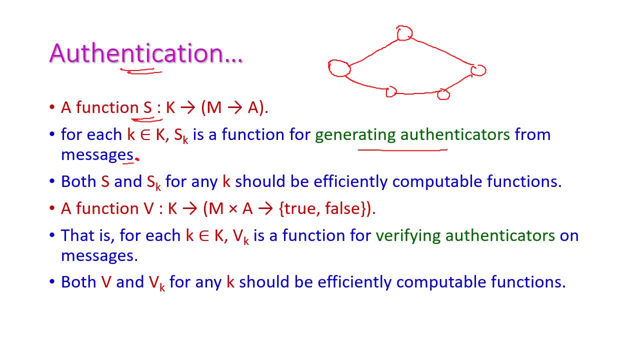 a separate authentication. that is, only the authorized users can access this particular network resources, or only those people can share the messages between each other. for that we need to test whether these users are authorized users are not. okay, this is called as authentication. okay, see, for each user there is a separate authentication.